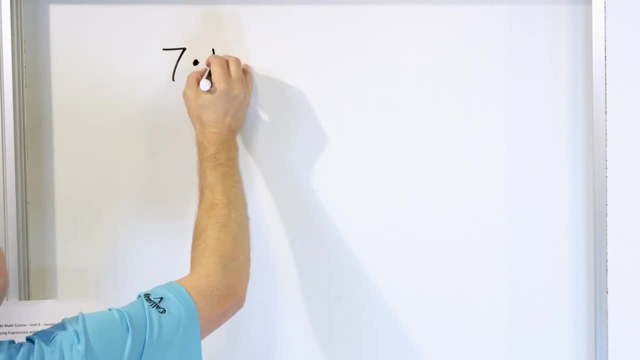 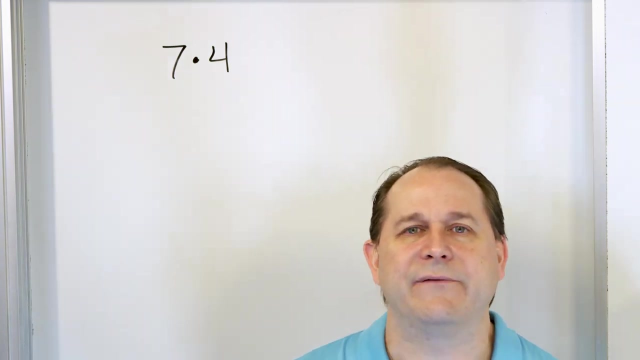 let's say that I tell you seven times four and I'm going to ask you: is this an equation or is this an expression? All you have to ask yourself is: does it have an equal sign? Well, I don't see any equal sign. I mean you might say, yes, seven times four is going to equal 28.. You know? 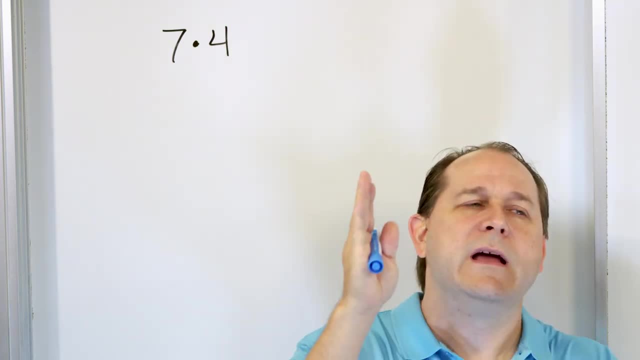 that in your mind, but there is no equal sign on the board. There is no left-hand side of the equal sign and right-hand side of the equal sign. So it's not an equation, because there's nothing equal to something else. This is just a calculation. Seven times four is a calculation. We call it an. 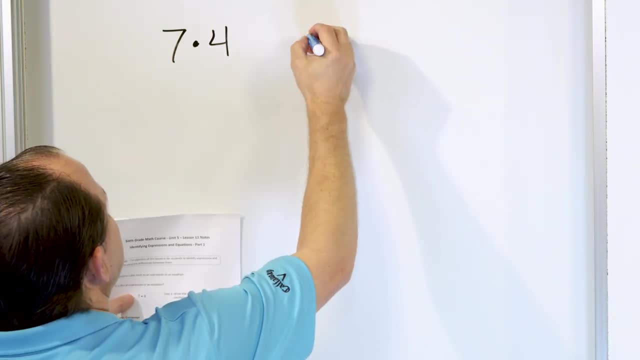 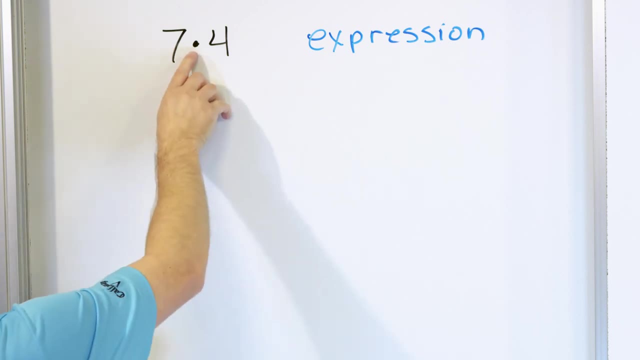 expression in math, right. So there's no equal sign. So this is an expression, right. Expressions can have numbers. They can have add, subtract, multiply, divide. Expressions can have exponents, Expressions can have fractions, Expressions can have decimals And expressions can have variables. 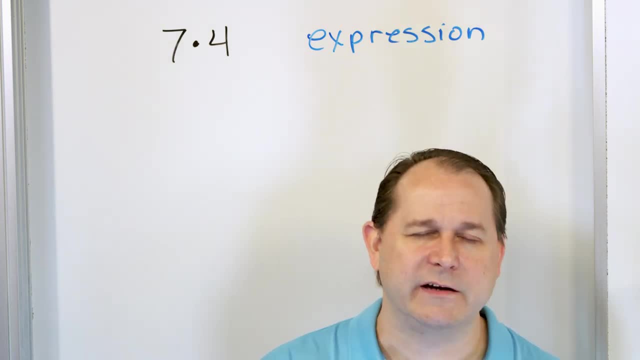 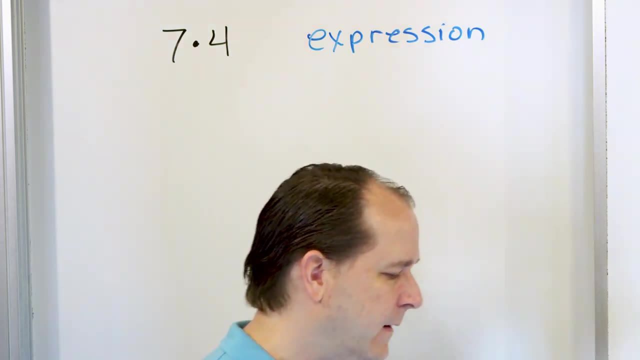 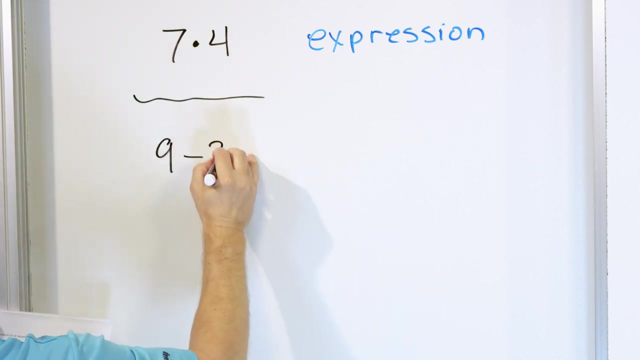 too. Letters, basically, And basically, if it's not an equation, it's going to be an expression, some sort of calculation happening somewhere. In this case, the calculation is just a multiplication. All right, now let's take the next example. Let's say that I tell you, nine minus three is equal to. 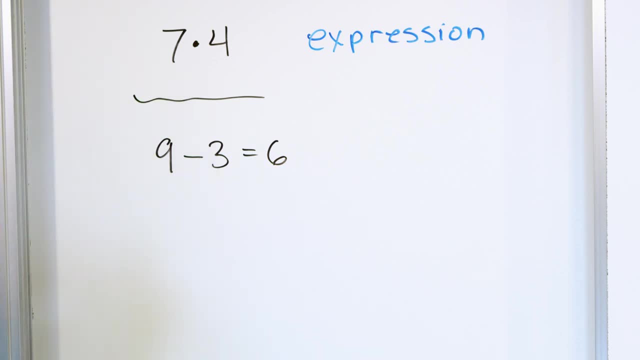 six. Is this an equation or an expression? Well, the only thing you have to ask yourself is: does it have an equal sign? Yes, it does. Equation means equals, So something is equal to something else. There's something on the board. There's something on the board. There's something on the 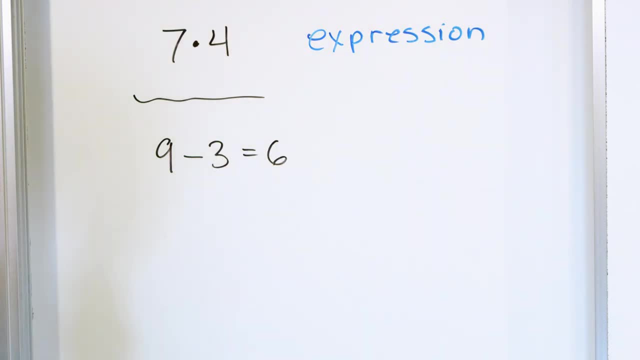 left-hand side of the equal sign And there's something on the right-hand side of the equal sign. There is an equal sign. So this is an equation. You know a lot of students when they hear about equations, they think, oh wow, that's so hard, Equations are so hard. Well, this is your. 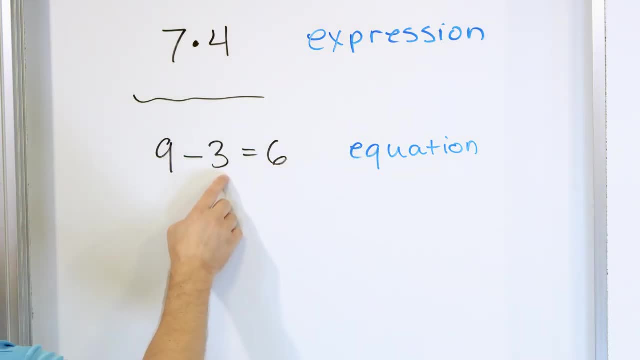 first equation. It's so simple, right? All it's saying is that nine minus three. well, just calculate this right here. What is nine minus three? It's six. So what you figured out is on the left-hand side of this equal sign. this calculates to a number of six, And the right-hand side is also a six. 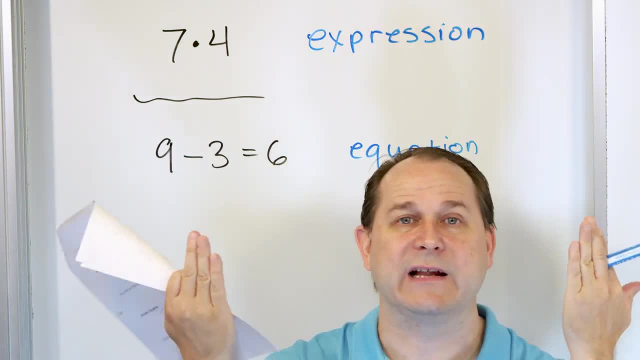 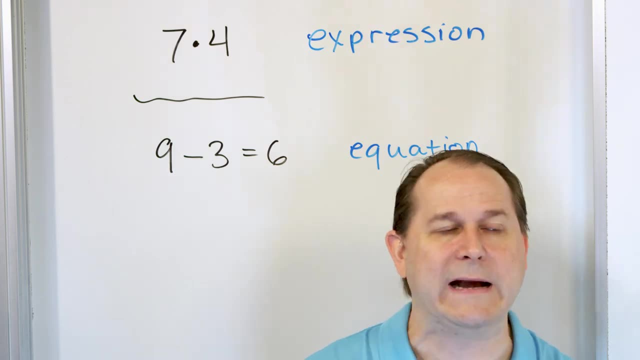 So the left-hand side and the right-hand side both calculate down to six And that means they can be joined with an equal sign, because the left-hand side is exactly equal to the right-hand side. This thing on the left, whatever it calculates to be, must come out to calculate to whatever's on. 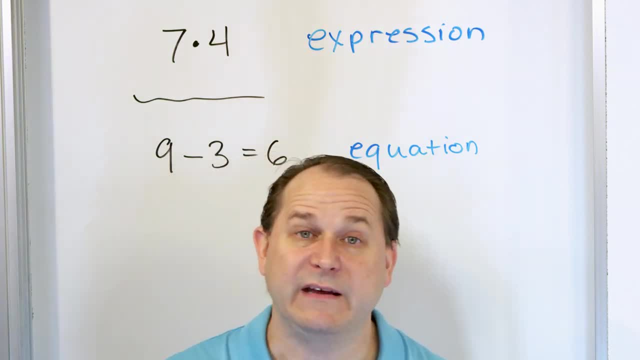 the right in order for this equal sign to be valid, Because equals means equivalent, exactly the same value on both sides. So if there's an equal sign, it's an equation, And of course the left-hand side should compute to be equal to whatever is on the right-hand side, And then what you have here is: 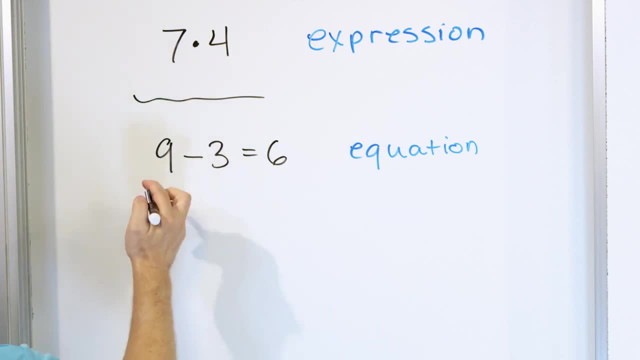 an equation. If there's no equal sign like above, then there's nothing equal to anything else. It's just called an expression. All right, let's take a look at the following: What about? 48 is equal to 12 times four. Is this an equation or an expression? Well, you look at it and say: 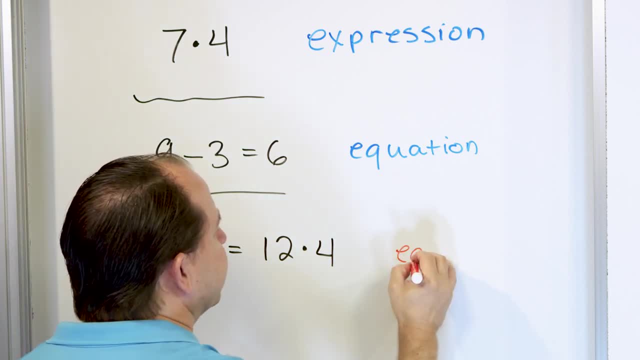 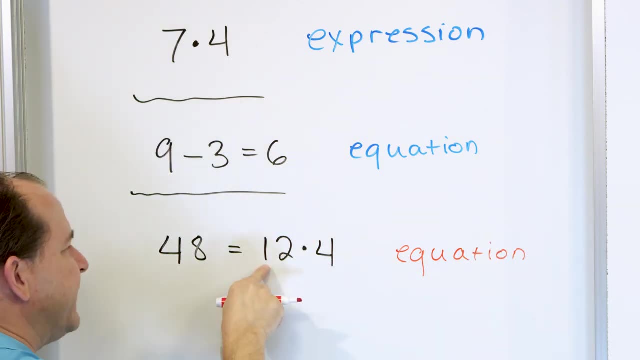 well, it's an equal sign, So it's an equation. See how simple this is Equation And you can double check and say: well, is this equation valid? What we're saying on the right-hand side is that- notice if I cover the equal sign up, this is an expression by itself, It's just. 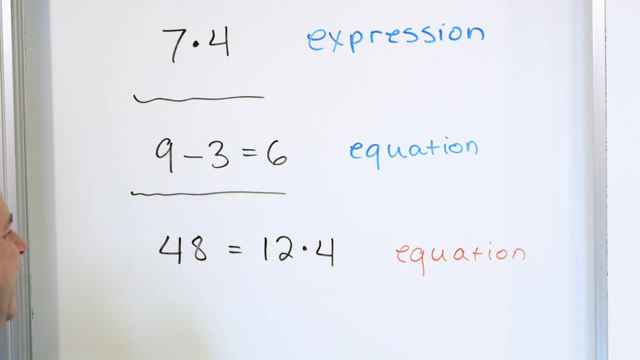 a calculation 12 times four calculates to be 48.. So what we're saying is: the right-hand side computes to 48.. The left-hand side is 48. And because they're the same, they're joined by an equal sign, because they're equivalent, And that is what we call an equation. All right, very simple. 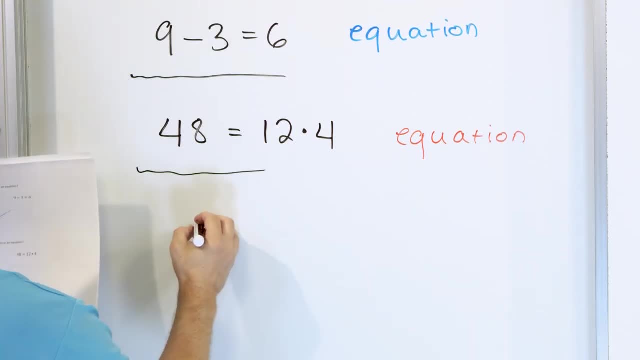 All right. what about the following? What about x plus 14?? x plus 14.. Is this an equation or an expression? Well, is there an equal sign? I don't see an equal sign anywhere, right? I just see a variable plus a number. right? Don't let the 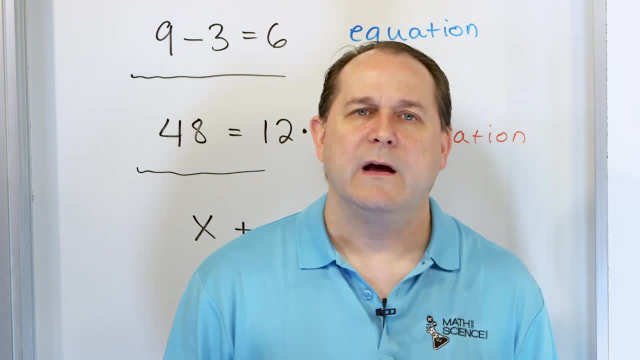 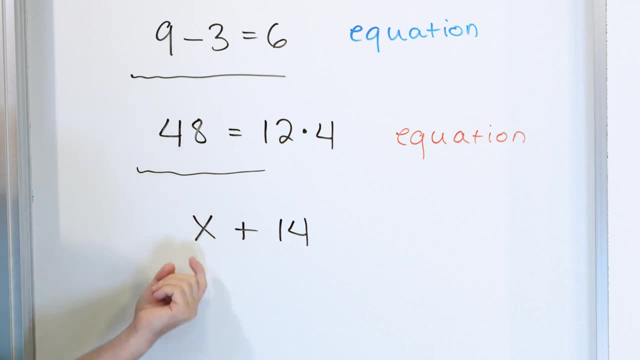 idea that a variable is here. scare you Remember a variable. a letter is just a placeholder. x is going to be something, x is maybe 1, or x might be 2, or x might be 10, or x might be. 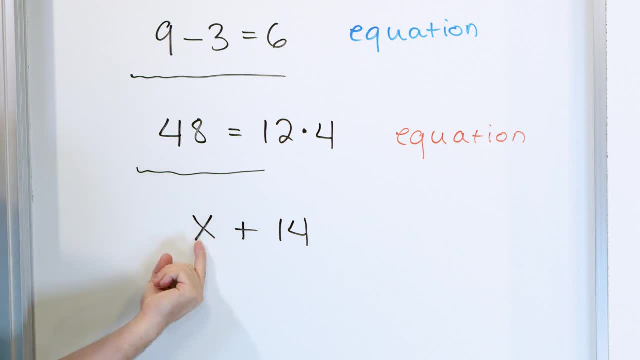 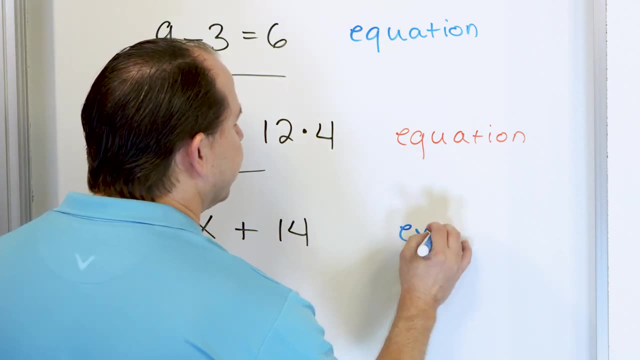 you know 0, or any other number that you can think of, 5.5. But it's just some number. but is this an equation? Do we have an equation? I don't know what it is. So the character n. 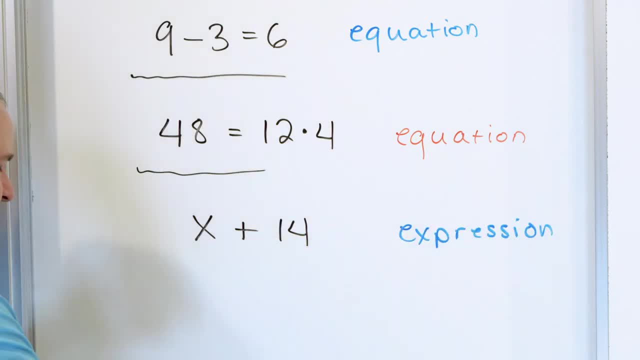 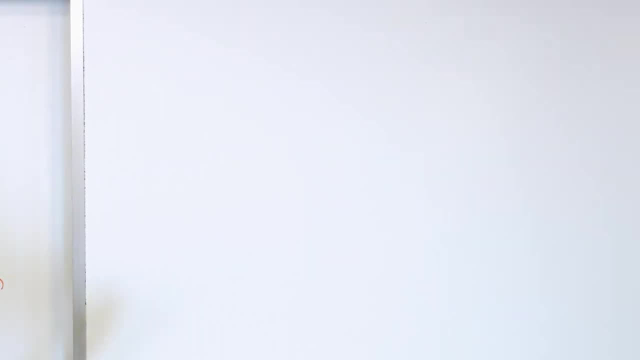 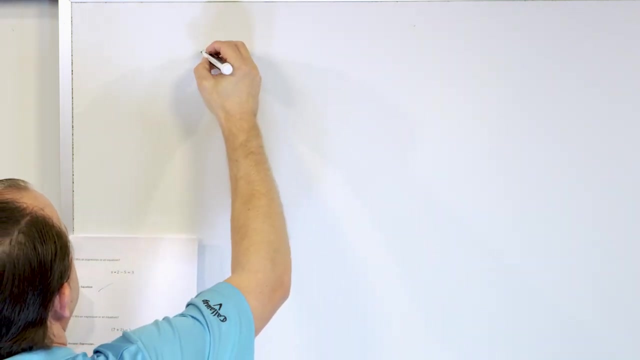 and then x equals 1, and x is 20.. Now what you're probably thinking is: well, in the math world, if you just take the vector and multiply it by 2, then you can get to the equation. Well, here's what I mean. Well, if you don't know what it is, then you can't learn anything. right, So let's move along to the next problem. Let's talk about n. multiplied by 2 minus 5 equals 3.. All right, is this an equation or an expression? Well, let's look at this problem now and see what's in it. 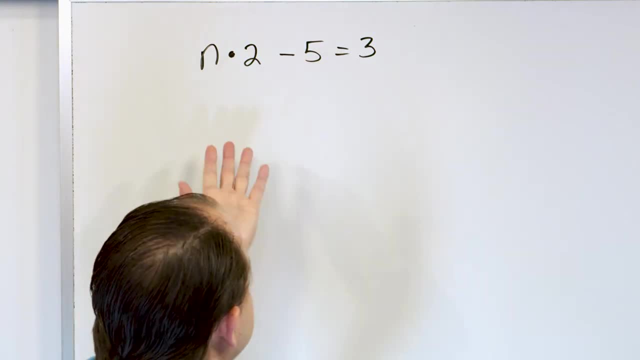 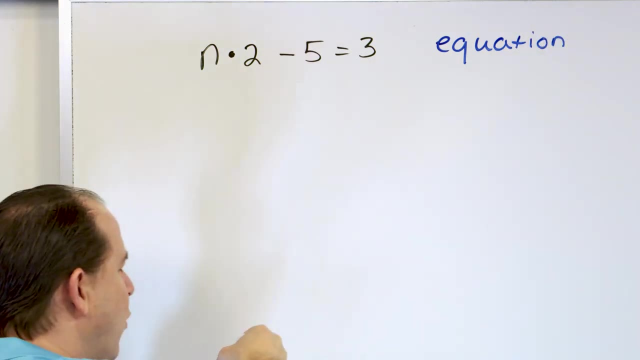 or is this an expression? Well, you can see that there's an equal sign. so immediately, without doing anything else, you know it has to be an equation. so put down equation All right now, whereas before, remember- this variable can take on any value. 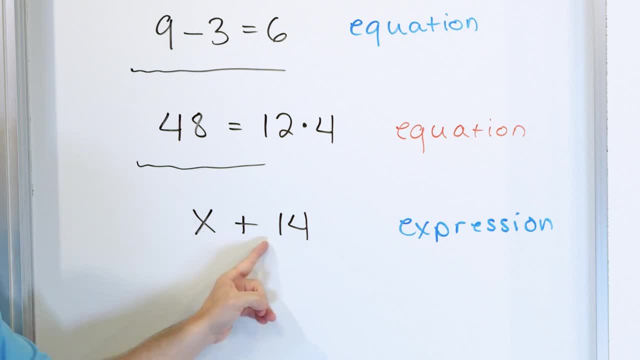 If I put zero in here for the value of x, then zero plus 14 will be 14.. If I put one in here, then one plus 14 will be 15.. If I put two in here, I'll get a different answer. 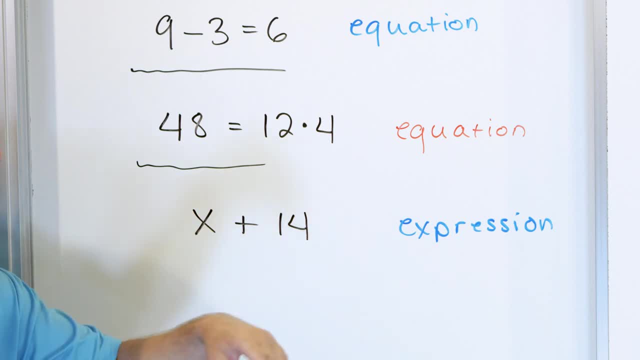 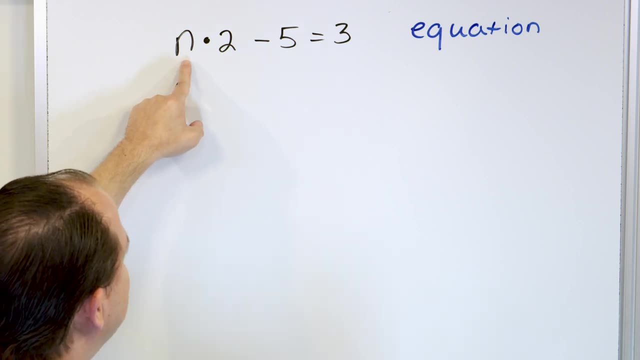 If I put five in here, I'll get a different answer. If I put 17 in here, I'll get a different answer. So, no matter what value I put in for the variable, I'll calculate something new. But in this case I have a variable. 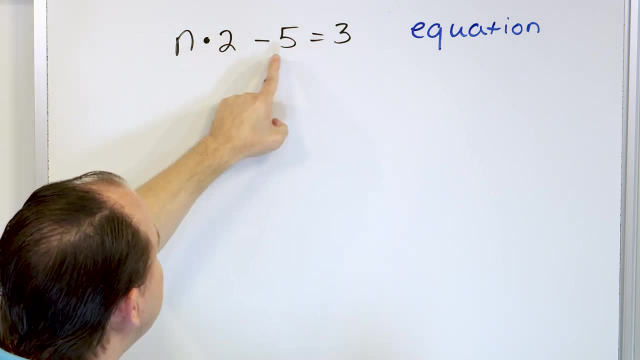 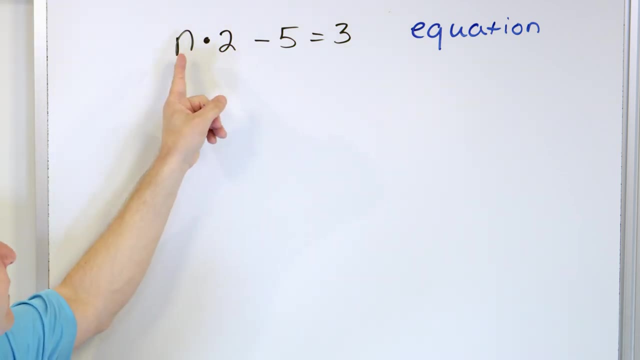 and it's equal to something else. So, because it's equal to something else, there's actually only one value that works for this variable. to make it equal, Let me say that again, There really is only one value of the letter n that really can work in order to make. 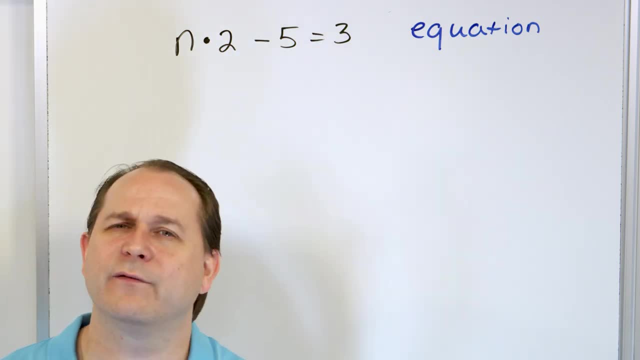 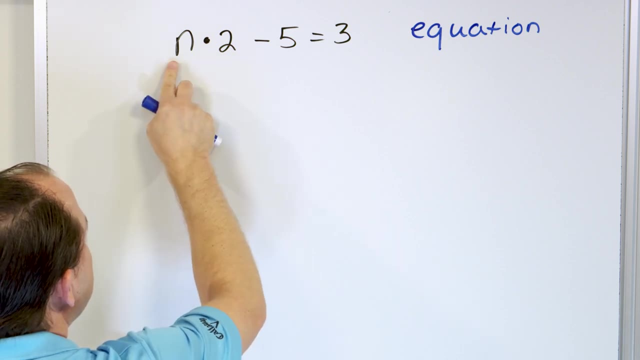 the left-hand side equal three. So let's just, since this one's so easy, let's just think through it. What if I put zero in here? Zero times two? This would make this whole thing zero, And then it'd be minus five. 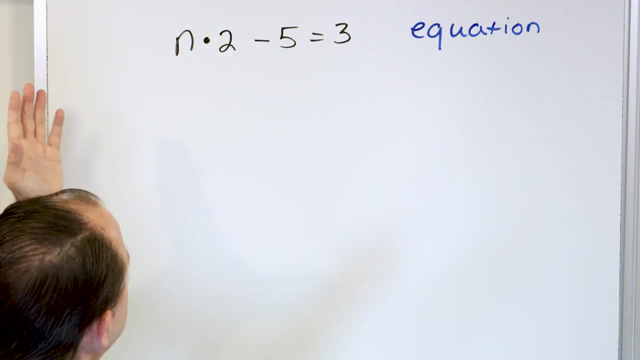 And that certainly is not equal to three. So the value then cannot be zero. What if I put one in here? One times two is two, And then two minus five? that's a negative number. That can't be three. What if I put, I don't know, let's say three in here? 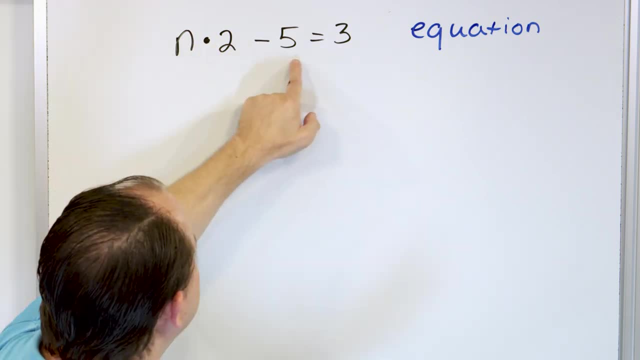 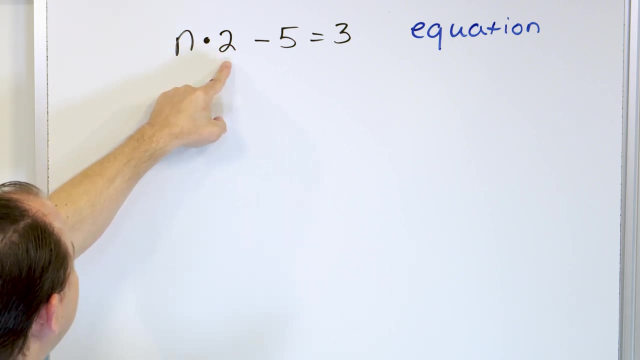 Three times two is six. Once I do that, six minus five, that's one. That can't be a right value. Let's try one more. What about four? Four times two is eight, And then, if this is eight minus five, that would be three. 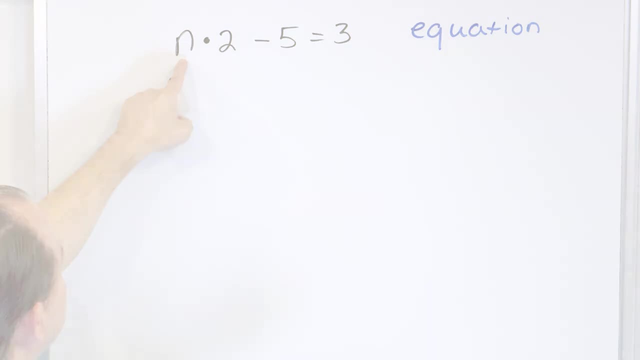 So, bingo, that means that this value right here has to be four. The value of this variable has to be four. If we pick zero or one or two or three, or if we skip over four to five, to six to seven, then no matter what we get when we use those other values. 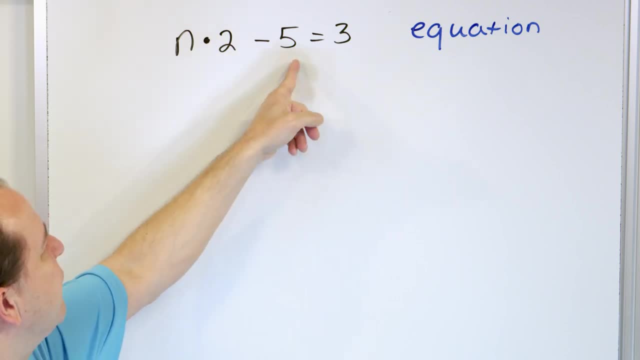 of the variable n, we're gonna get something other than three on the left. So if we get something other than three, it means it's not equal to three, So it's wrong. This is really the value of an equation. here is when we have an unknown in the equation. 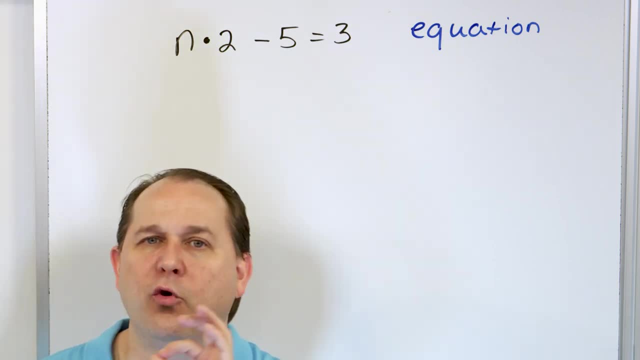 to figure out what the unknown is. Maybe you write an equation down to talk about the temperature in this room or the weather pattern over the ocean. or you write an equation to figure out how fast you're going when you reach Mars and your spaceship. 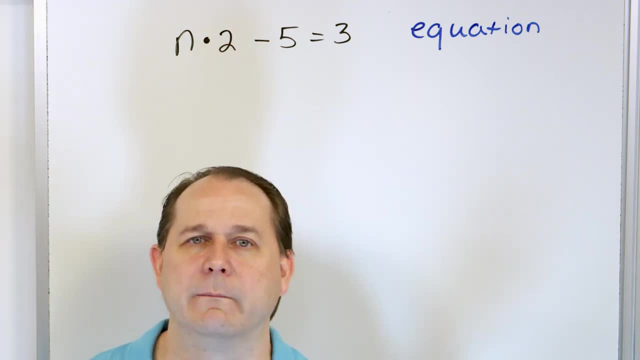 or you write an equation to talk about the black holes and how they form And you don't know the value of the of the value. But that's the point of the letters in your equation. then you use the rules of math to figure out what they are. 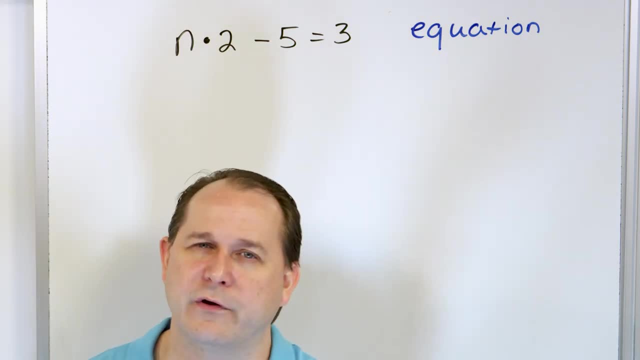 Now for this equation. we guessed and we got it right. but as we go further, we will learn how to solve these equations without guessing, because the equations get way more complex than this. But I just want you to know that an equation is just something with an equal sign and if 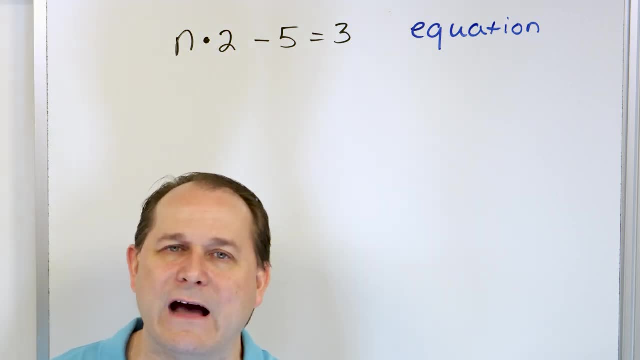 your equation has a variable. it just means that there is a value of that variable that will make that equation true, and the other values of the variable- they won't work. So later on we'll be solving equations to find out the right value that works. that's what an equation really is. 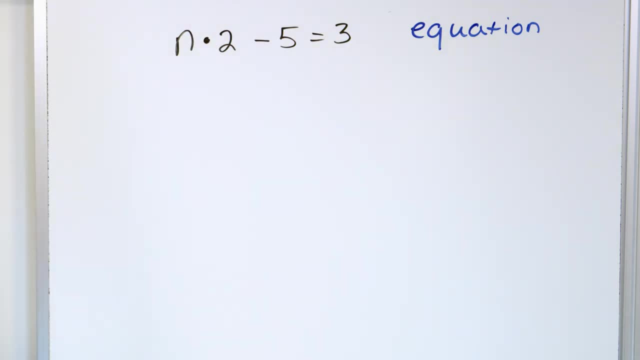 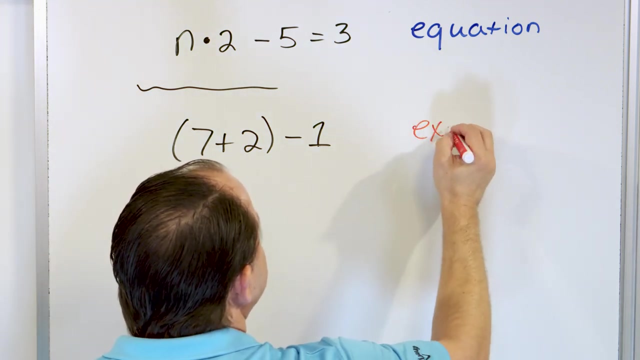 that's what they're for, okay, All right, that was a little bit of an aside, but a really, really important aside. Let's take a look at the following: seven plus two minus one: is this an equation or an expression? I don't see an equal sign, so this is an expression. 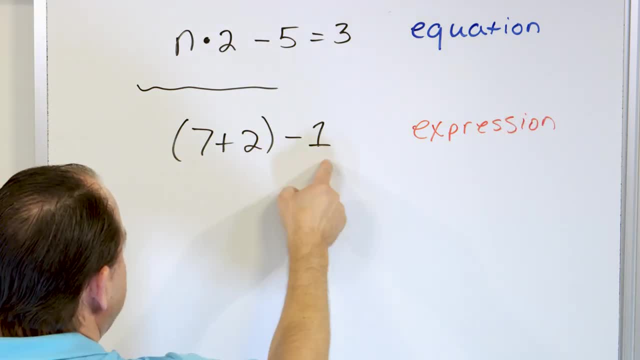 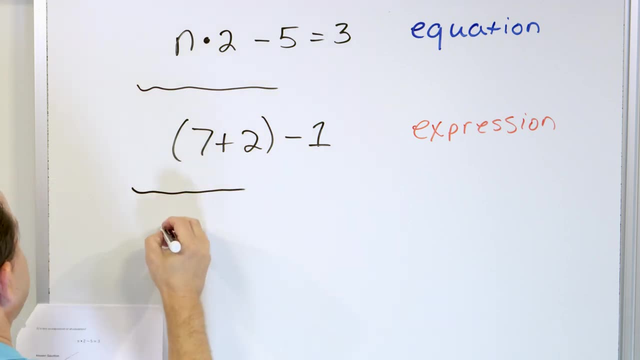 Right now. of course, I can calculate this. if I want to, I can calculate this and minus one, I get the number, but it's not an equation because it's not equal to something on the right hand side. All right, what about 48 divided by 2 plus b? has a variable in it, but there is no. 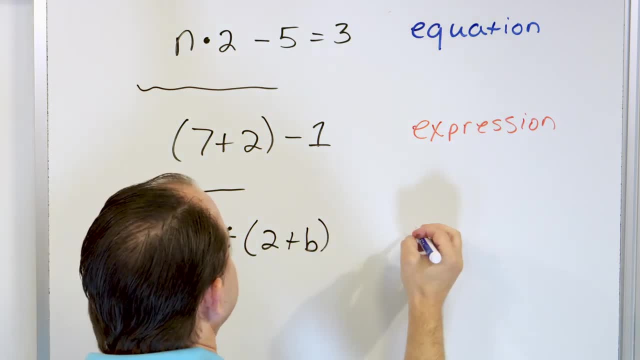 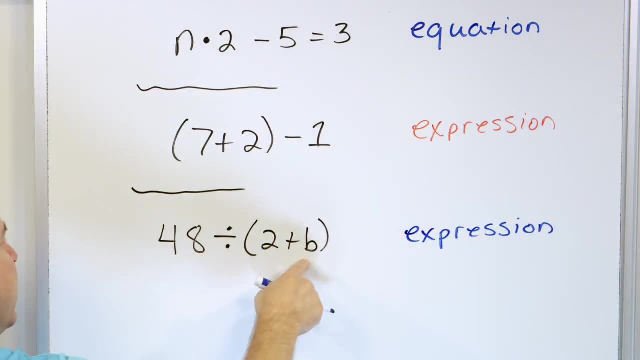 equal sign. No, equal sign means it's not an equation. this has to be an expression. So if I put different values of b in here, you know I'll add it to 2 and I'll take 48 divided by that I'll get new answers. if I put b is 0, b is 1, b is 2, b is 3, I'll. 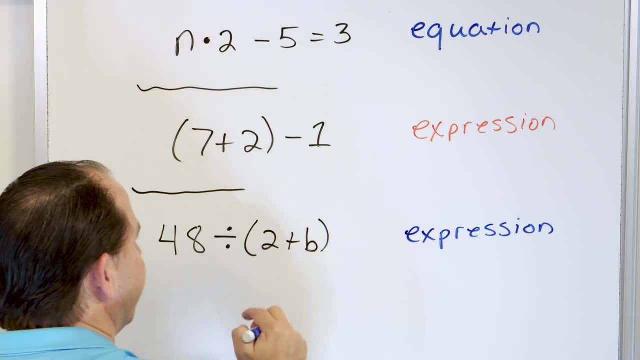 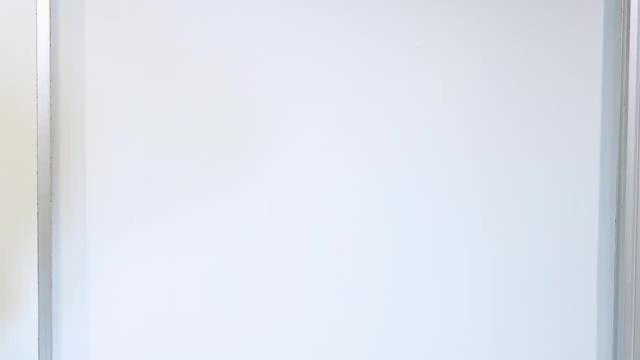 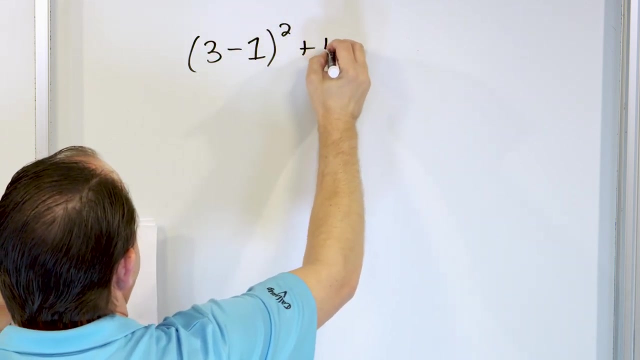 get different answers, but it's not an equation because it's not equal to something. there's no equal sign there, All right, all right, we're getting close to the end here. Let's take a look at 3 minus 1, squared plus 5 equals 9.. Is this an equation or an expression? 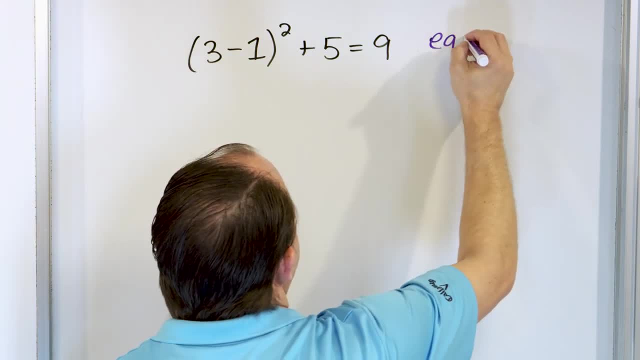 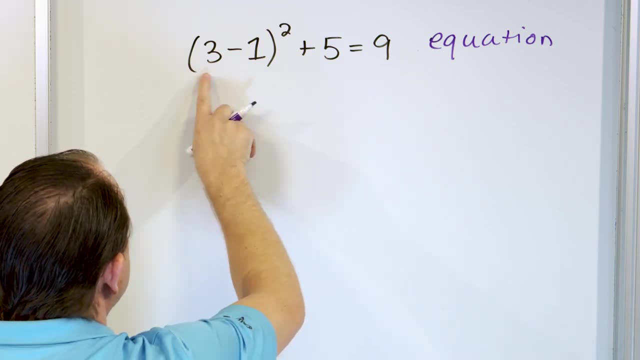 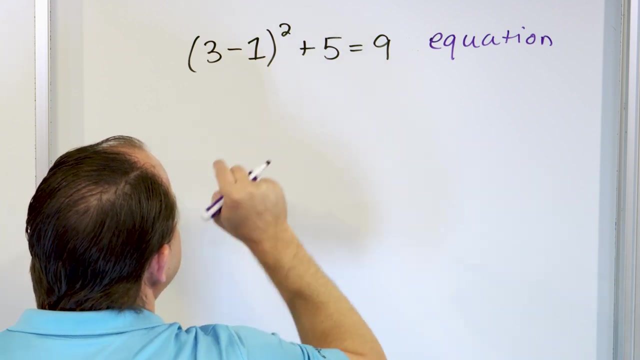 Well, I see an equal sign, so it has to be an equation. All right, let's take a look at it. just for giggles In the parentheses: 3 minus 1 is 2, so this makes 2.. 2 squared 2 times 2 is 4, so this whole thing makes 4, and then 4 plus 5 is 9,. 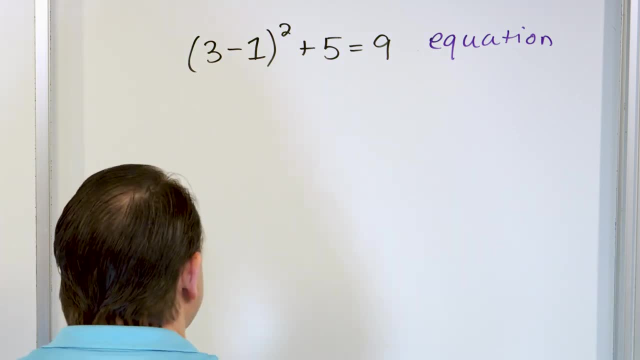 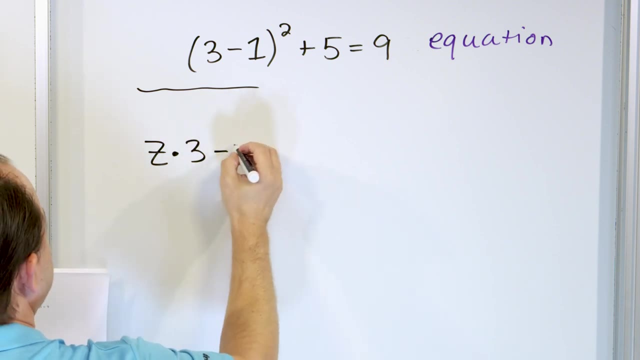 so this is an equal sign that is valid. that is an equation. All right, let's move along. What about z times 3 minus 4 plus 5 is equal to 24.. Is this an equation or is this an expression? Well, I see an equal sign, so it has to be an equation. 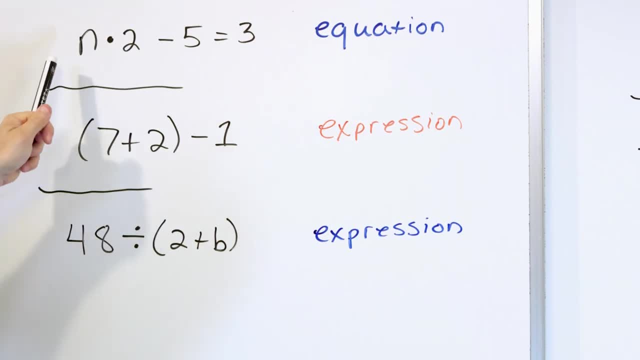 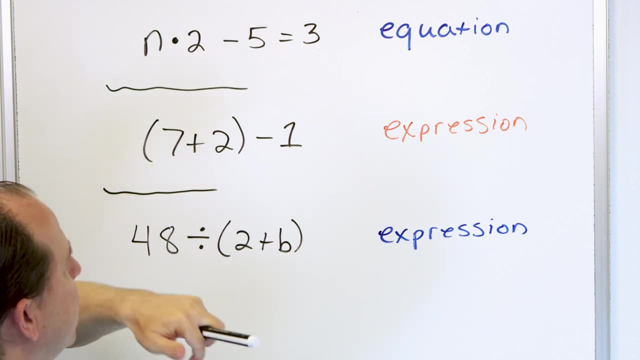 Right now, much like before. notice before, when I gave you an equation here that had a variable, we started guessing values and calculating what, what the correct value of the variable is. that makes it true. Here you could do the same thing, but notice, it's a little more complicated. so 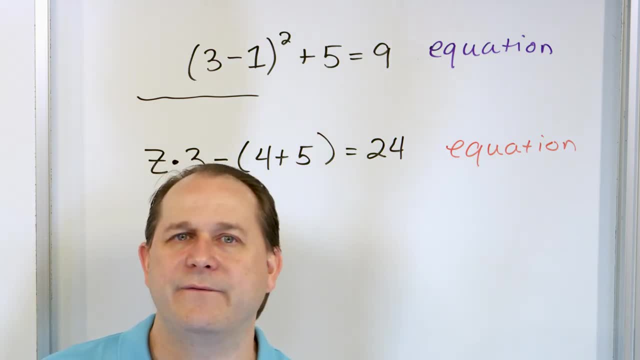 it's going to take more work. So guessing like that to find the value of the variable, that works. guessing over and, over and over again, it doesn't really work. for more complex equations it would be guessing forever. So as we go through math, I'm going to teach you. 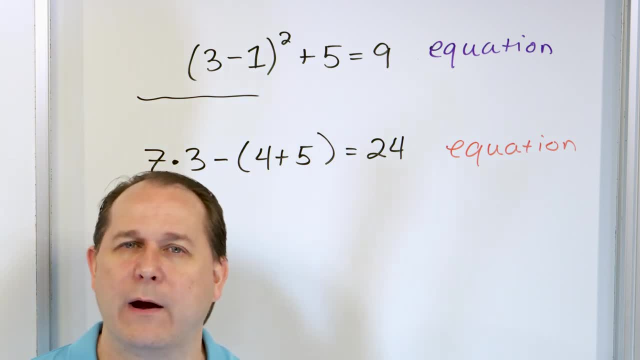 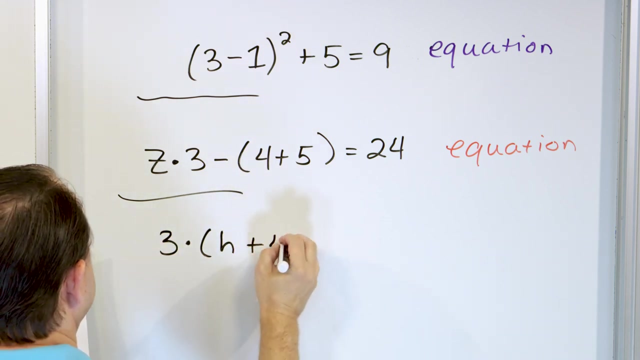 how to solve these things and find the right value of the variable. that works without guessing and there's rules involved, but you'll get used to the rules, like anything else, and you'll get good at it. All right, what about 3 times h plus 4 divided by- uh, whoops, divided by what? divided by 2.. 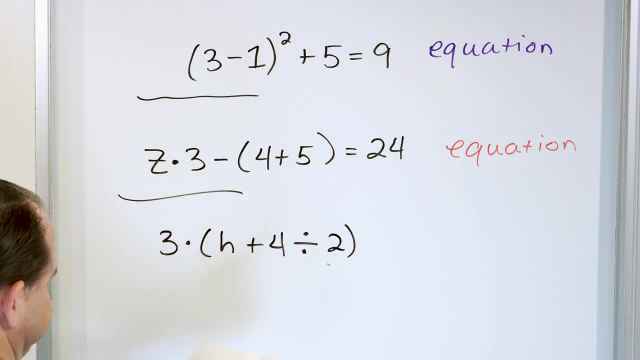 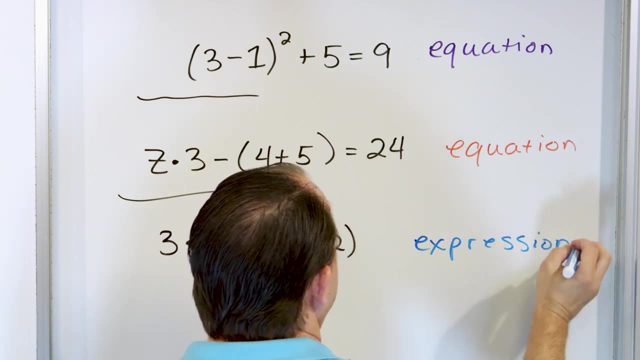 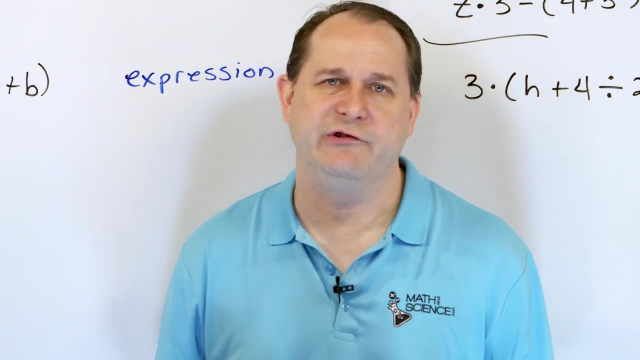 All right. is this an equation Or is this an expression? I don't see any equal sign anywhere, so this is an expression, All right. so the goal of this was really twofold. The first goal is to tell you what an expression is and what an equation is. In a nutshell, an expression is another way of saying calculation. 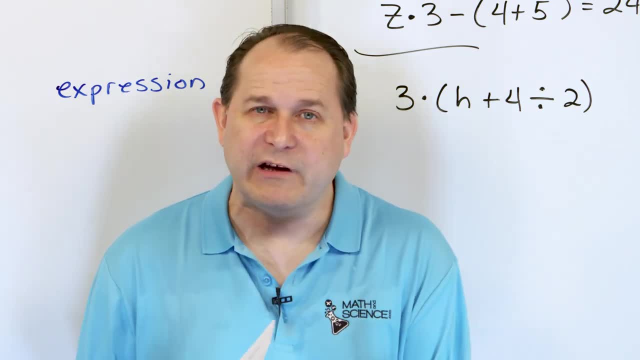 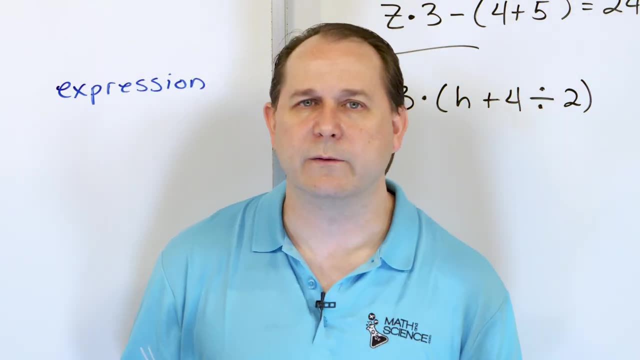 in math, right, when you calculate something right. An equation has an equal sign. The left-hand side of the equal sign must be the same in value whatever is on the right-hand side of the equal sign. That's why they're equal. So we want to learn the difference. basically, if you see an equal sign, we call it an equation. 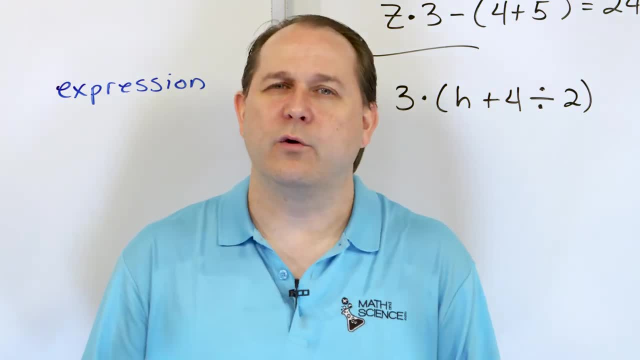 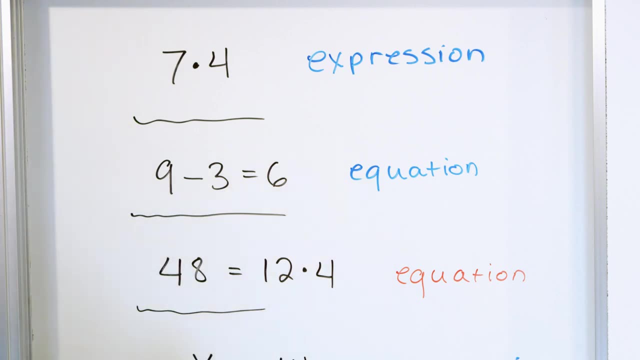 anything else, you basically call it an expression. and then we also went down the rabbit hole a little bit about what it means to have an equation. anyway, We talked about the simplest of equations. see that this is an equation because they're an equal sign. The right-hand side computes to 48, the left-hand side is 48, yes, that's. 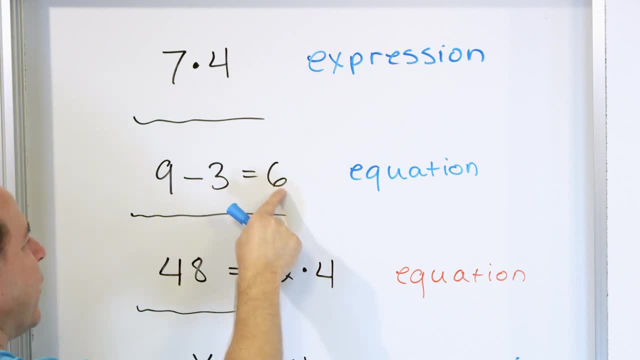 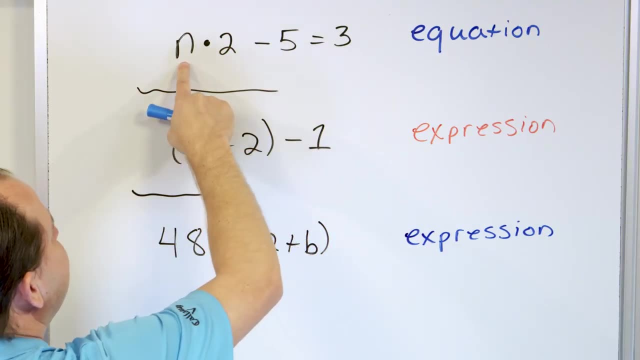 equal, so it's an equation. This computes to six and the right-hand side is six. that equal sign's valid equation. Now, when you get to an equation that has a letter involved, it just means that you stick different values in for this letter. then the calculation that happens you're going to get. 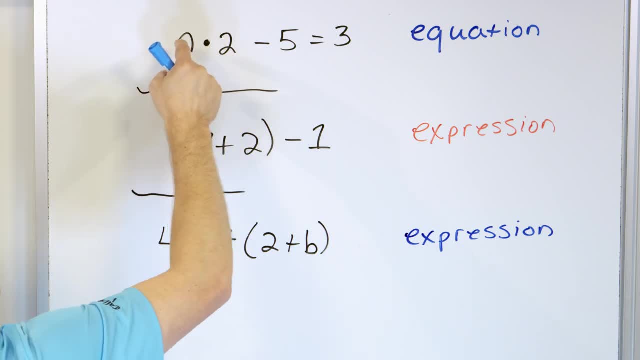 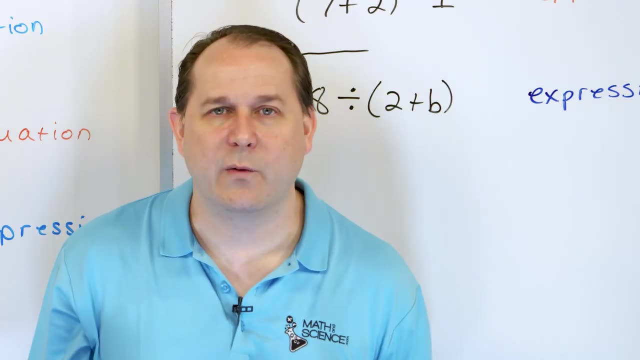 different answers And you have to pick the right value of the variable to make it equal- the right hand side when you calculate it. And that process is what we call solving the equation. Now, here we haven't really solved it. we kind of guessed and convinced ourselves right that this has to. 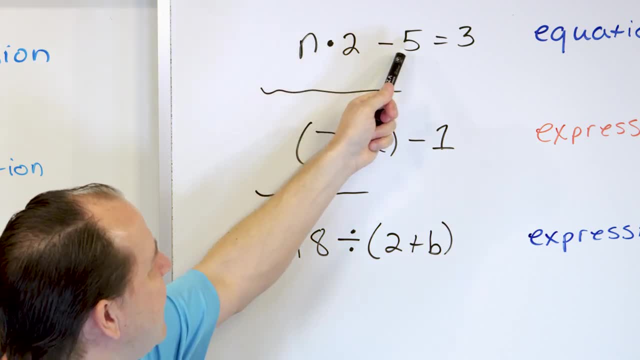 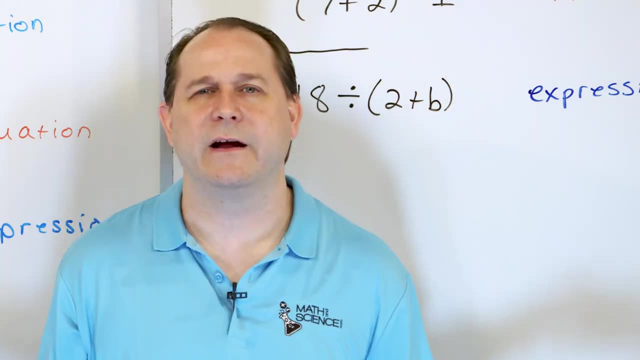 be four. n has to be four, because four times two is eight, And then you take eight minus five and then it's three. that value works. But as we go farther in math, we learn how to solve these things, And there are many, many, many kinds of equations, from very simple equations related to 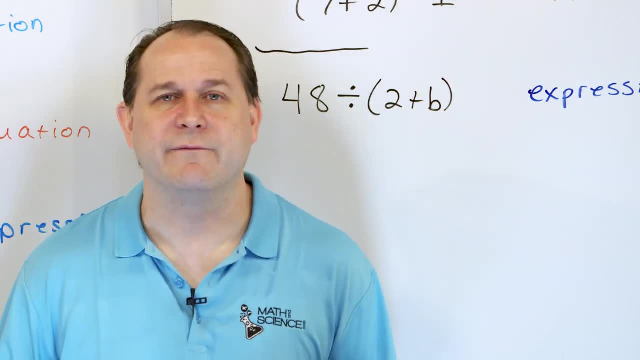 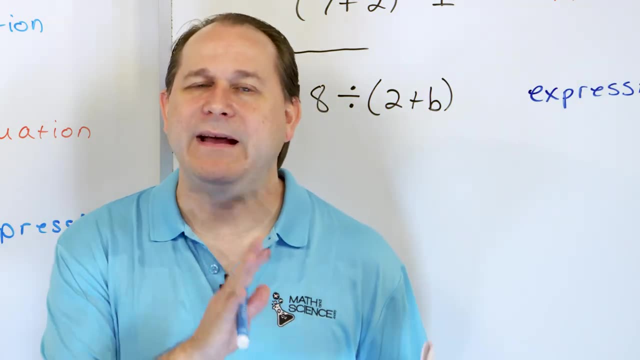 distance and money and time to very complex equations involving gravity and black holes and electromagnetic waves and radiation. they get very complex, But the basic idea is the same: you have an unknown, you have something you want to learn about and solve for, and we write an. 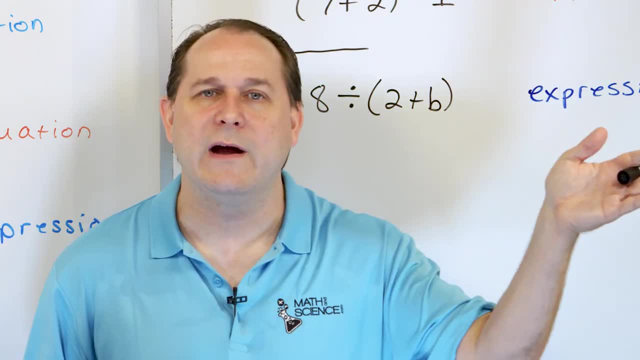 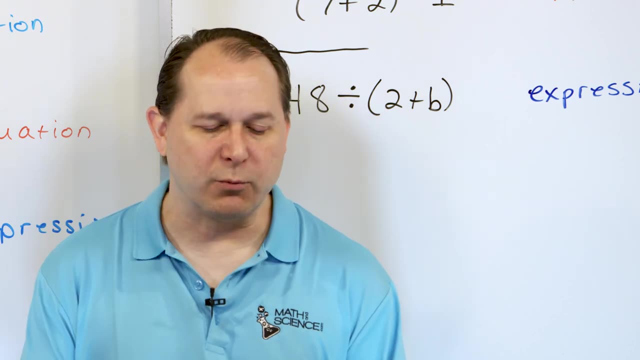 equation and we solve it. So that's the direction we're going. That's where we're heading. So I'd like you to finish solving all of these yourself And, when you feel like you understand what's happening, go on to the next lesson. we'll get a little more practice to wrap. 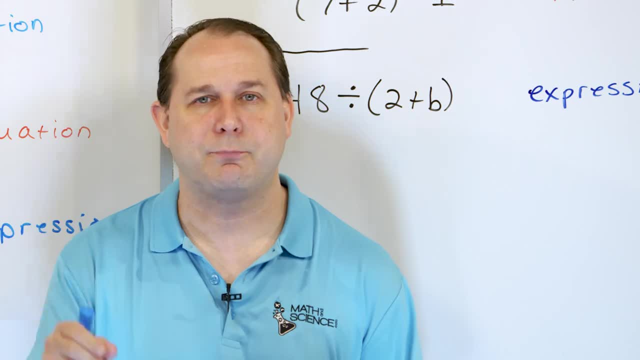 up the concept of identifying equations and expressions.